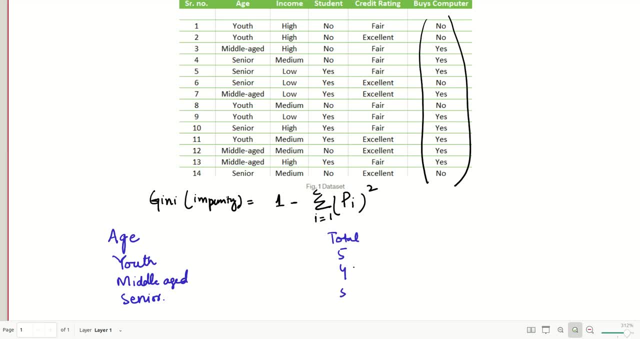 instances and senior has five instances as well and in class. yes, in no, we will categorize them as well: youth and youth and senior. we have four instances and senior has four instances and in one, two, three, three times it has appeared in class. no, it is one, two, three. 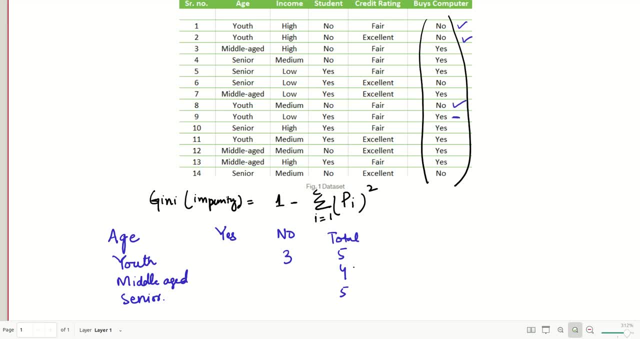 right, and two times it has appeared in class yes. similarly middle-aged: four times it has appeared in class yes, in zero times. in no senior has appeared one, two, three time and yes and two times in no. so let me calculate the gene index now for the feature age. 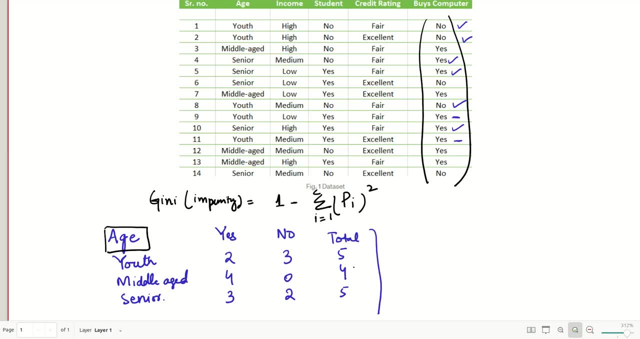 well, first of all, let me calculate the gene index for youth, when edge is equal to youth, by formula. well, the youth has appeared two times in yes to do I my five whole square, and three times it has appeared in no and total it has five instances. well, genie. 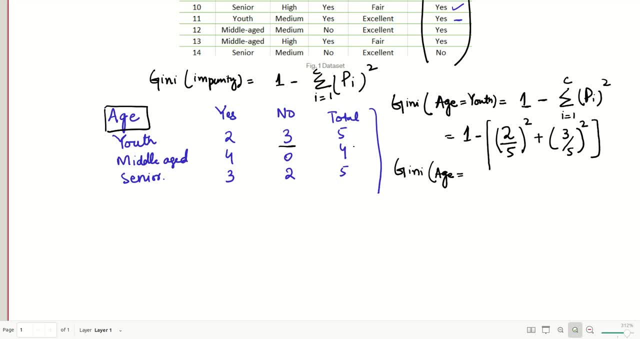 when edge equal to middle-aged you bar: yeah, yeah, yeah. and time times: it has appeared yes and totally. has four instances: 0, timing, no while terms: 2: position 1: yes, one, two, three times it has appeared in yes and total it has four instances. i need to mention: in 2 times it has appeared in no is four instances: 701. 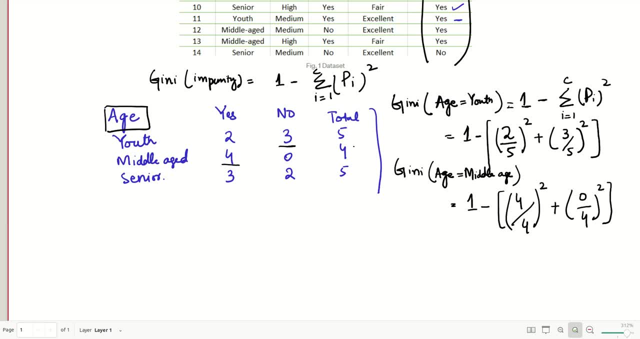 Walking. yeah, good, great, yeah, ญ. GIN index for edge equals senior equals 1 minus. when we put these values in the formula- this one, three times- it has appeared in yes. total instances five. two times it has appeared in no: total instances five. so these are the. 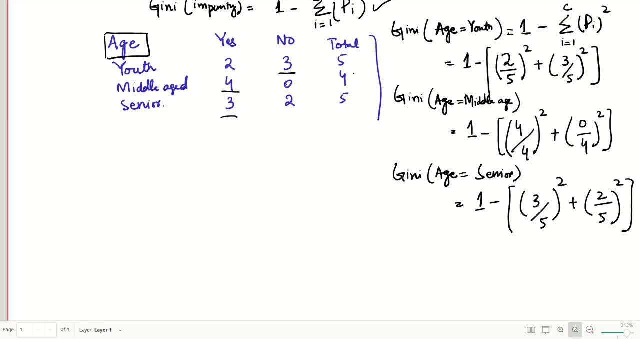 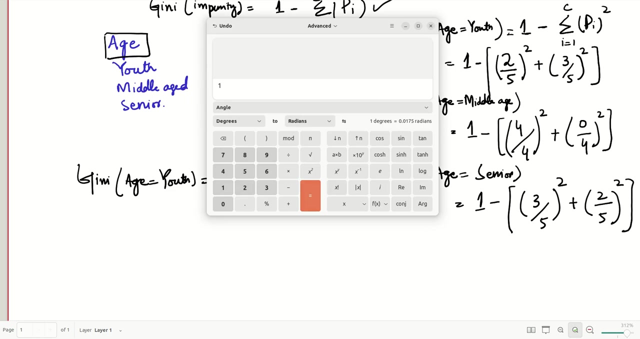 mathematical equations for the GIN indexes of the individual values such as youth, middle-aged and senior in the future age. now let me calculate the values of the individual values. we will get to the point. is the GIN of age equal youth is. let me calculate it using the calculator: 1 minus 2 divided by 5. 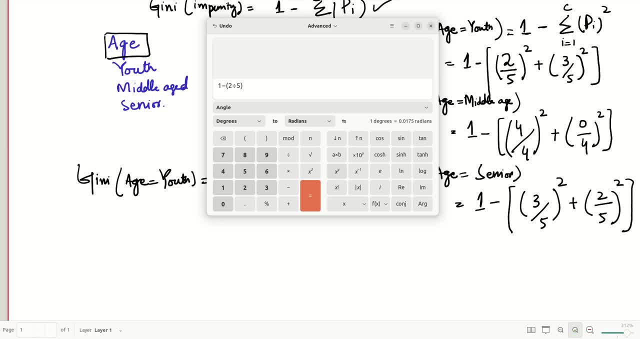 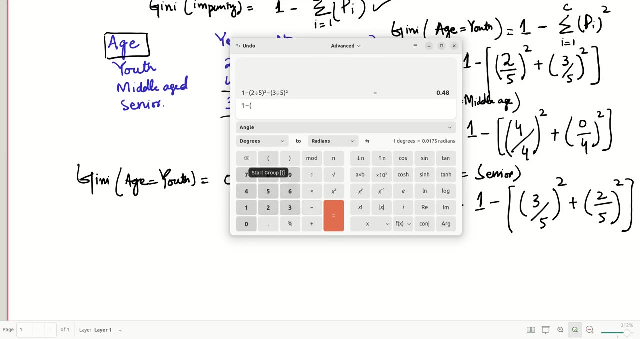 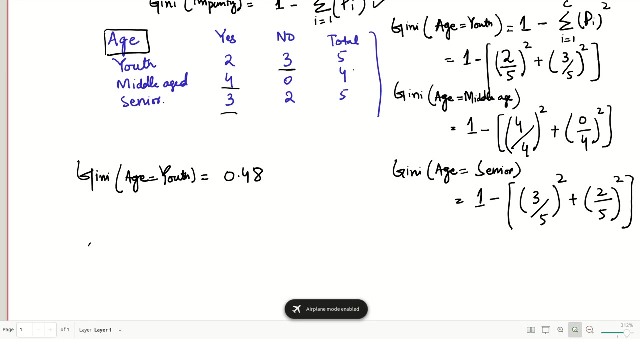 or hole. squared minus three, divided by five minus three, divided by 5, whole squared minus two, divided by 5, half, called square Again, the result is 0.48.. So Gini for age equal to senior, Then it is equal to 0.48.. 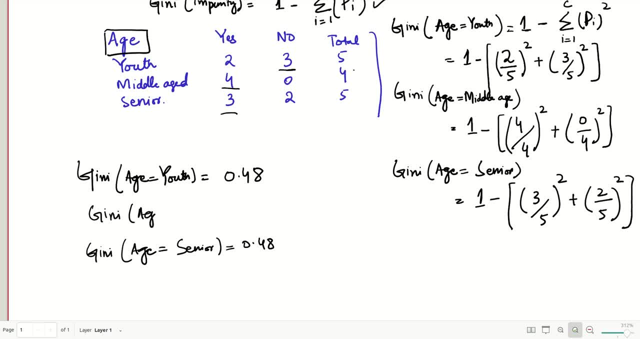 While the Gini index for age equal to middle age- Well, it is equal to, since this will be 0- and 4 by 4 is 1.. So 1 minus 1 is 0. Well, The Gini Value of the 0 indicates that there is no impurity in this value of the edge feature. 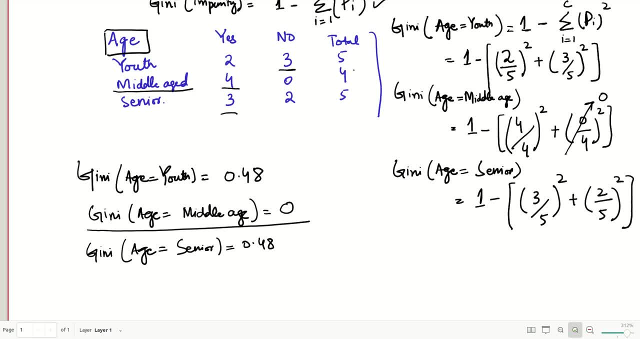 that is straight away. if middle aged is, if the value is middle aged, then the class is: you know, the class is yes, right, The target class is yes. So we calculate the Gini indexes of all these three values of the edge feature. We want to have the weighted sum of the Gini index on the edge parameter. 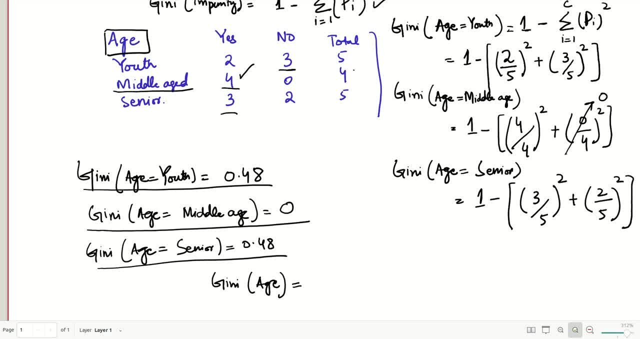 So the Gini index of the edge, the entire edge feature, equals 0.48.. In this case, edge equal to youth plus 0 plus 0.48.. But we we want to have the weighted sum, So the edge has 5.48.. 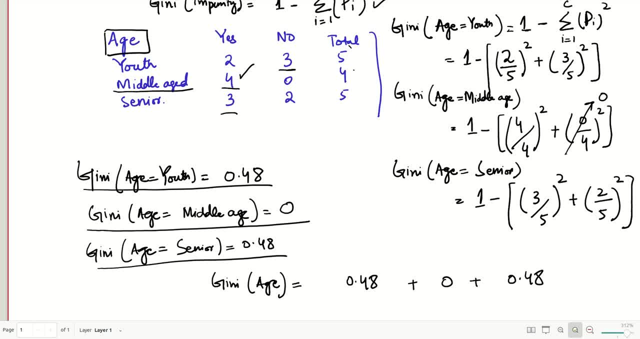 So When edge equal to youth, youth has 5 instances, So 5 divided by 14, total 4 instances are 14.. In this case, 4 instances for middle age, so 4 divided by 14, since it is 0, so it would: 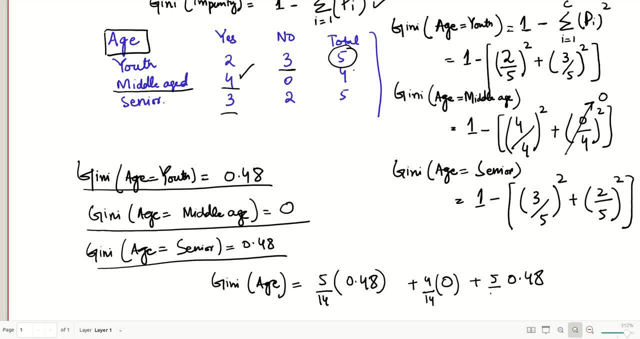 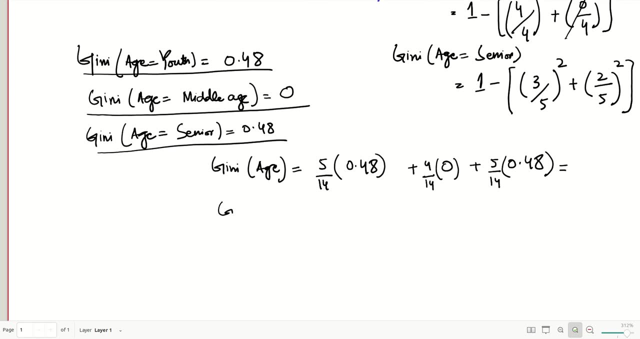 have no impact. And similarly 5 by 14: 0.48.. So When we mathematically calculate these values, So the Gini index for the entire feature would be the weighted sum of the individual indexes. So let me calculate it.